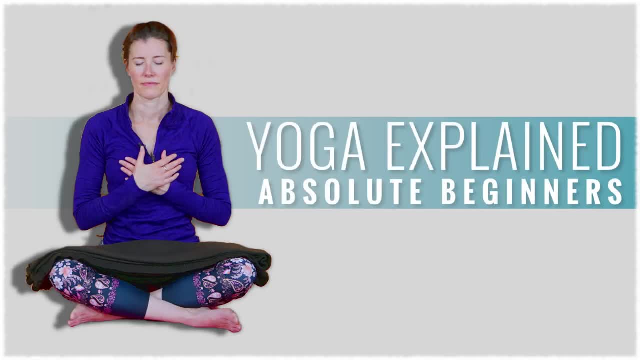 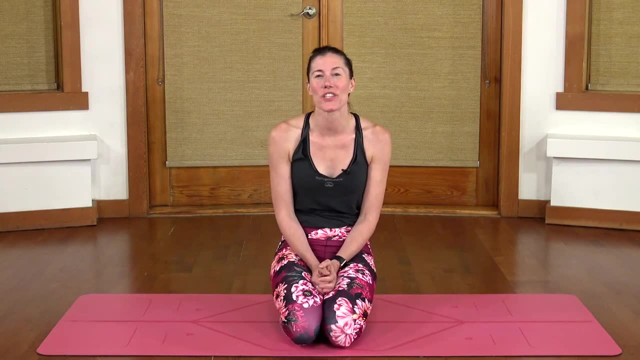 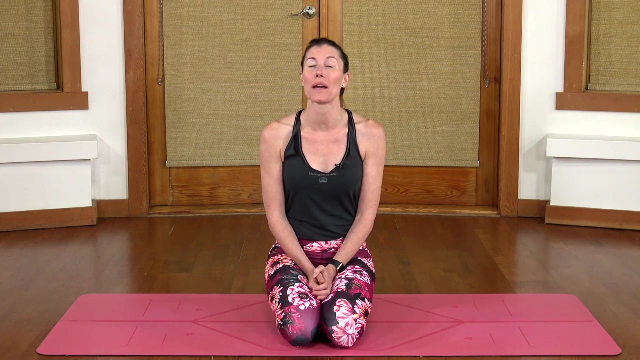 Hi, I'm Rachel with. Do Yoga With Me, and this is Yoga Explained, And in this video I just wanted to share some of my thoughts for those of you out there who might be a beginner or newer to the practice. So, first of all, sometimes yoga can feel intimidating. We see the Instagram poses. 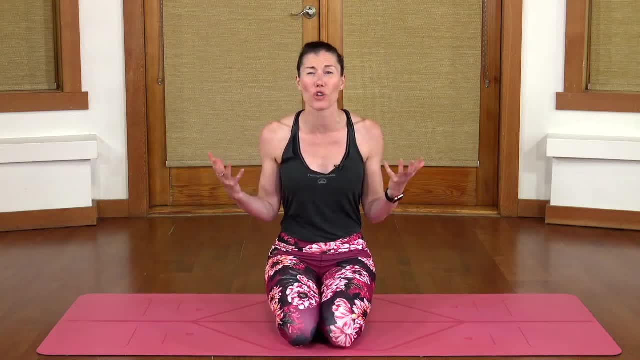 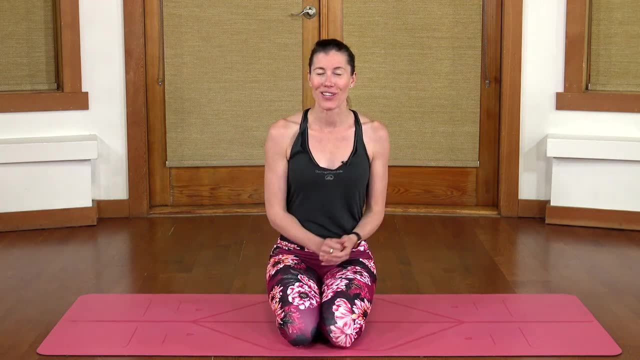 we see the fancy poses out there and it looks one like you have to be like super flexible and strong to do yoga in the first place, And I want to tell you that all of that is a lot of hooey. So you do not have to be flexible to do yoga. You do not have to be able to do fancy poses to do. 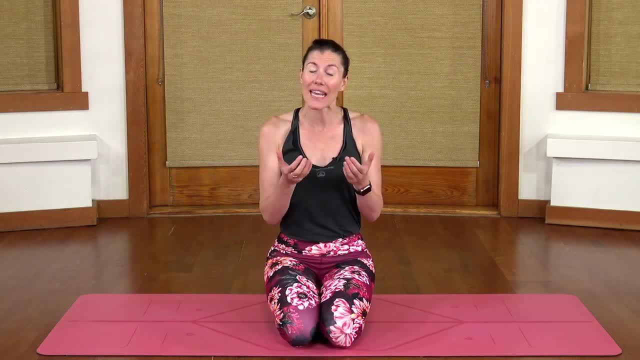 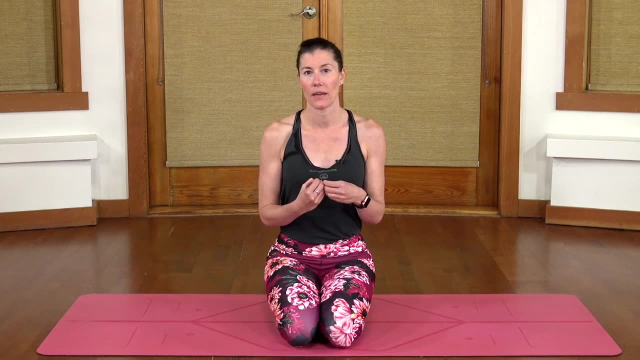 yoga. Yoga, ultimately, is really one about taking care of your body and yourself, And really the magic of the yoga practice is what it offers for your mind. So we do the physical practice, which is really wonderful, And then we do the physical practice, which is really wonderful. 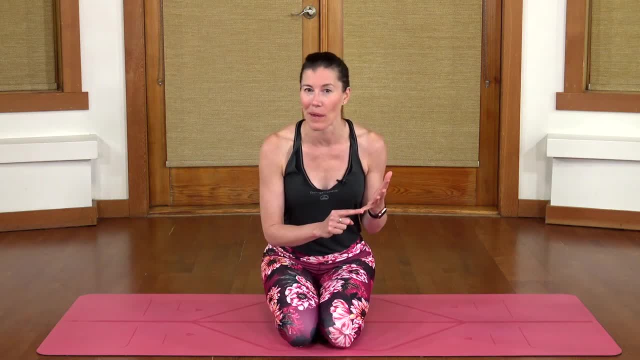 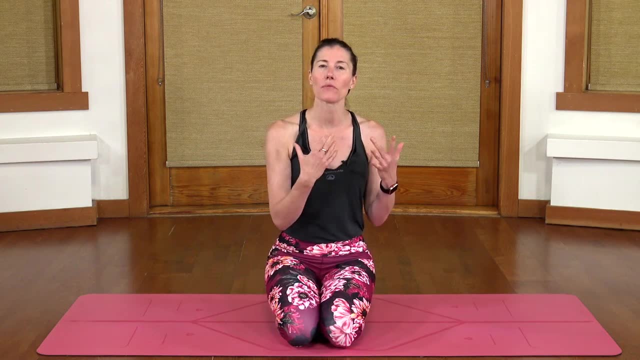 Because it helps us to stretch us out where we might be a little tight. It helps us get stronger where we might be weak. But the real jewel of the practice is that it gives us time to be with ourselves, And it also helps us do one of the best things that we can for our body, which is to calm. 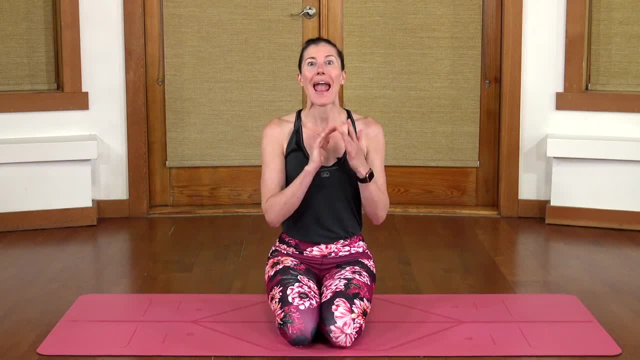 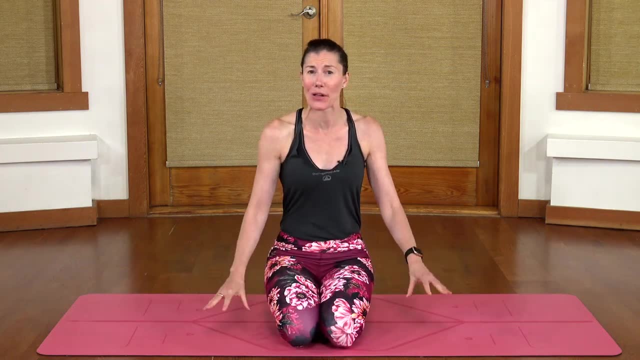 our nervous system and calm our mind. So anyone can do yoga. It doesn't matter Even if you have a mat. you don't have to have any particular kinds of fancy clothes to do yoga. You can do it in your favorite comfort zone, You can do it in your favorite place. You can do it in your favorite. 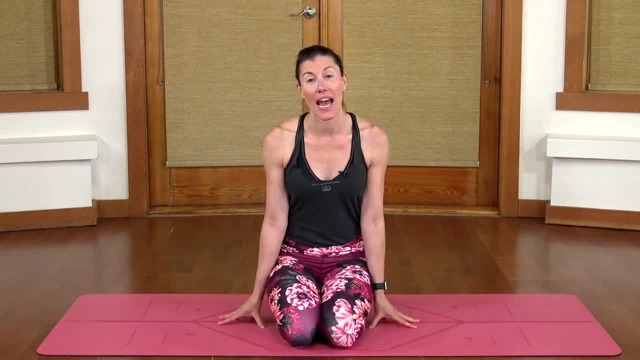 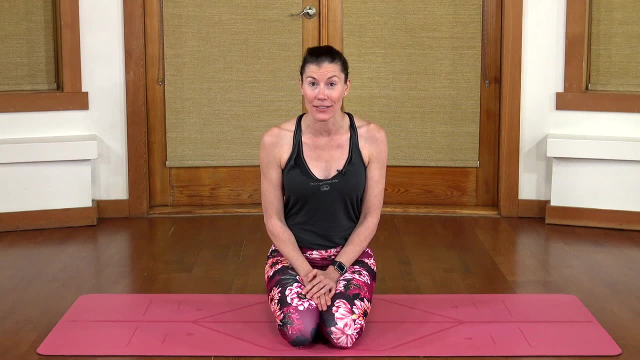 place. It doesn't have to be sweatpants. at home, Although a mat is nice to have, you can really use anything that won't let you slide. So I have done plenty of practices on my sister's living room carpet, for example, when I visit her. When you're doing yoga, you also don't need any fancy. 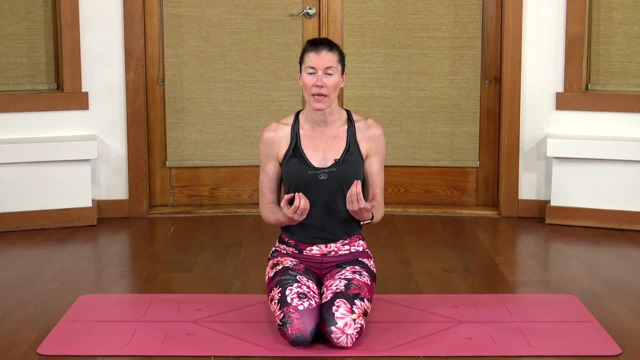 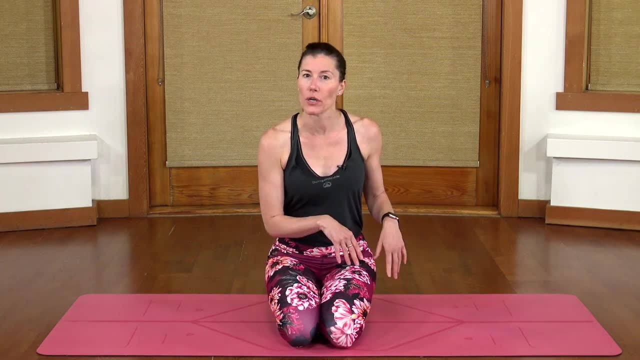 props. So if you're practicing with us at home and do yoga with me, you don't need anything fancy like you don't have to go out and buy things. If we're using blocks, you could use a couple of books. If we're using a strap, you could use a couple of books. If we're using a strap, you could. 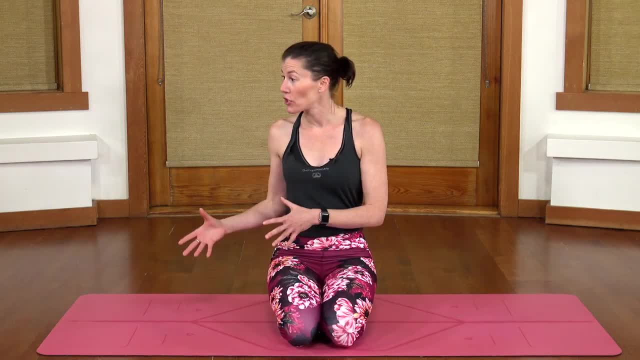 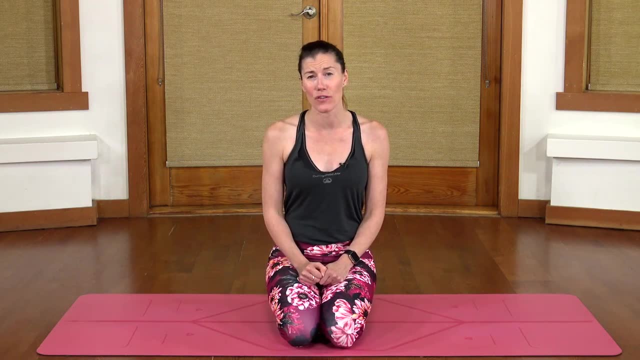 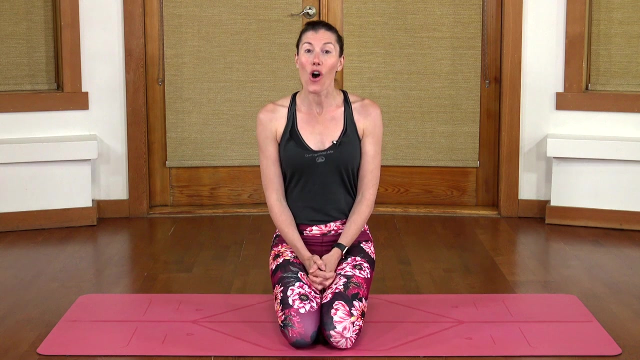 use a scarf or a tie. If we're using a bolster or a chip foam block, you could use one of your pillows or one of your sofa cushions. So there's nothing fancy that you need to do for the practice. Really. ultimately, it's just about you creating a little time and space for you And also.